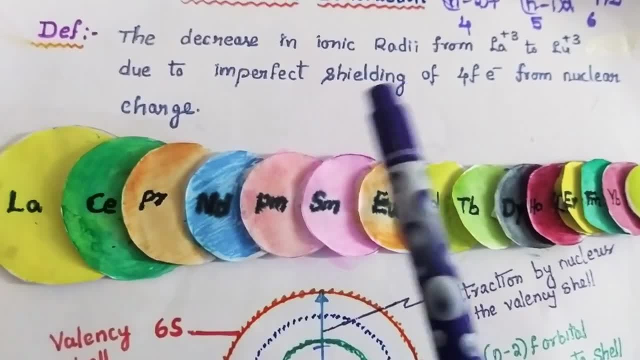 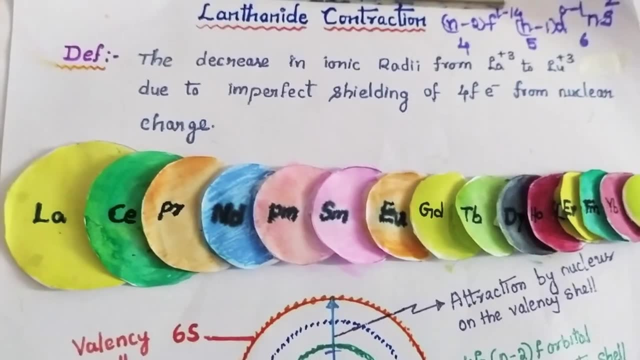 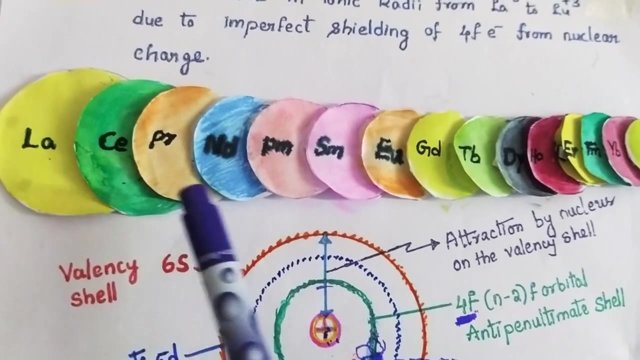 in ionic radii from lanthanum to lutetium due to imperfect shielding of 4F electrons from nuclear charge, is called as lanthanide contraction. The another way we can define this one as the steady decrease, the steady decrease in sizes of lanthanides with the 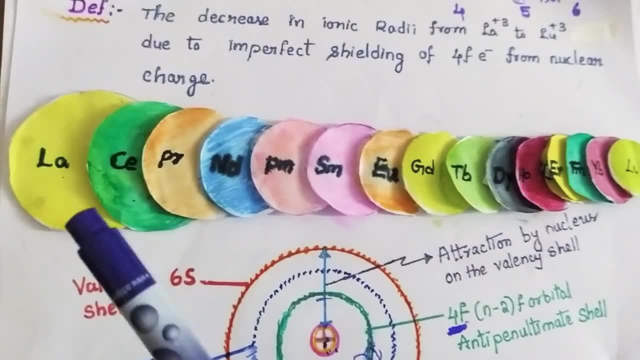 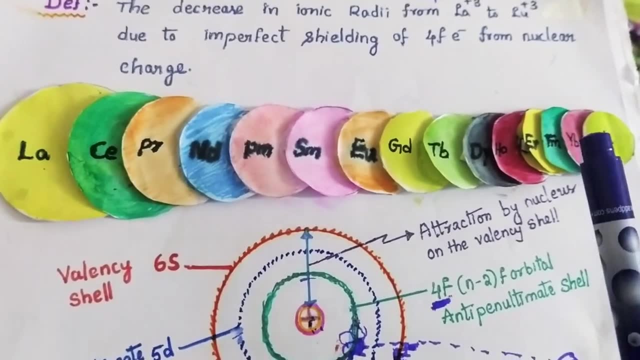 increasing atomic number is called lanthanide contraction. Here you can notice there is a regular decreasement of atomic sizes from lanthanum to lutetium, which is known as lanthanide contraction, and this is due to the imperfect shielding of 4F electrons from the nuclear 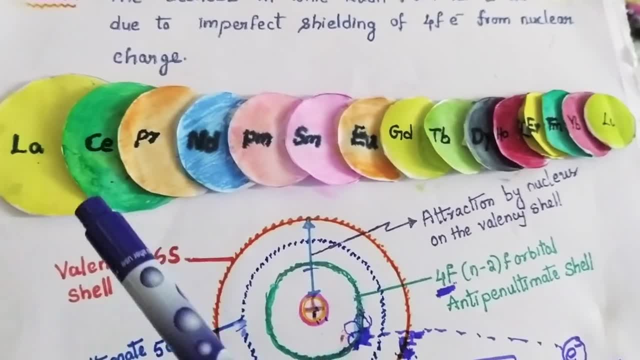 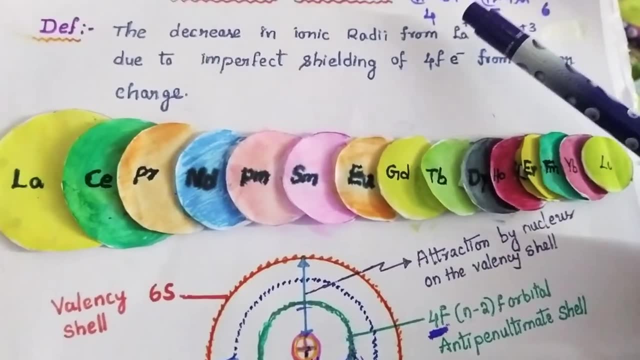 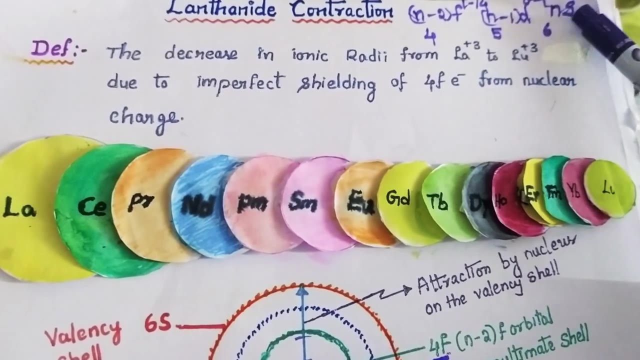 charges. So let's see what is the reason for the contraction of the lanthanides. If we notice the lanthanide, the outermost electron, that is general electronic configuration, is this one: As we know, that is N-2F1 to 14, N-1D0 to 1, NS2.. Here lanthanide is corresponds. 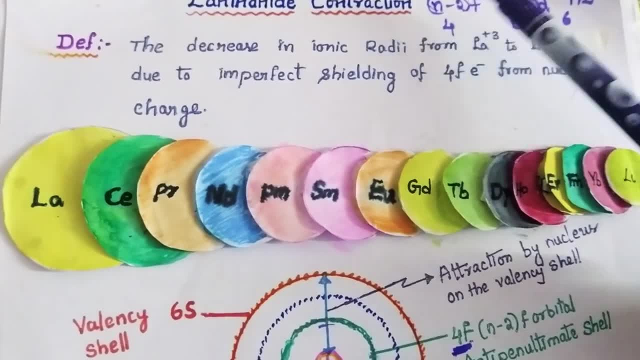 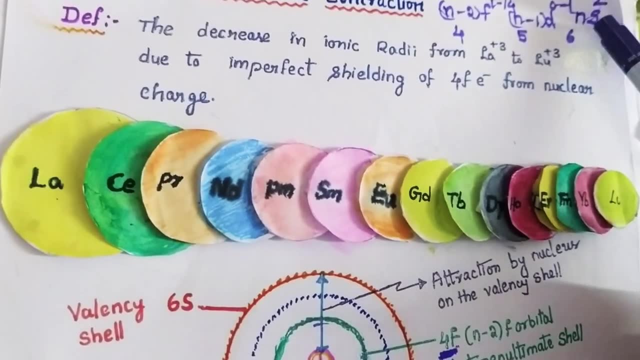 to the 6th period. substitute N equals to 6, so 4F1 to 14, 5D0 to 1, 6S2.. So notice here, students, carefully. The 6S2 electrons is common for all from lanthanum to lutetium. every nucleic is consisting. 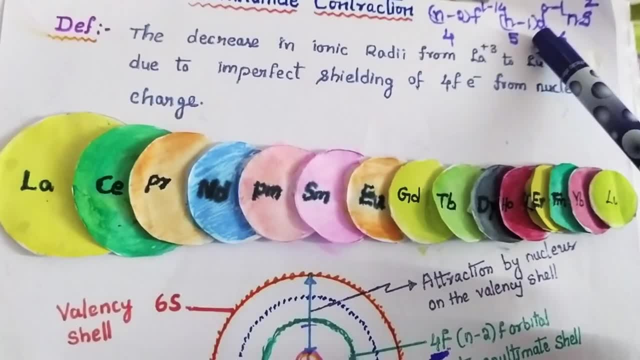 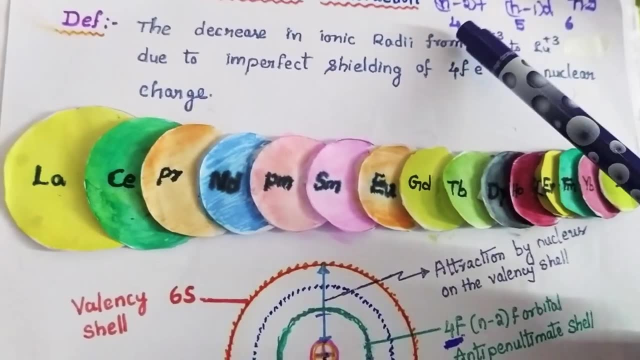 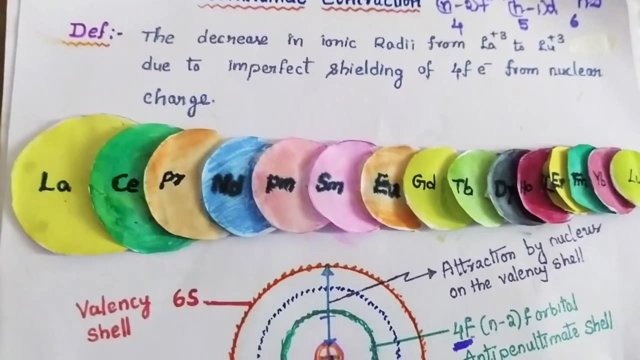 same number of S electrons And the D electrons there is a slight variation, that is D0 to R1, 1 electron difference is there? The only difference you will observe in the 4F electrons there is a large difference from lanthanum to lutetium, from 1 to 14 electrons. So if 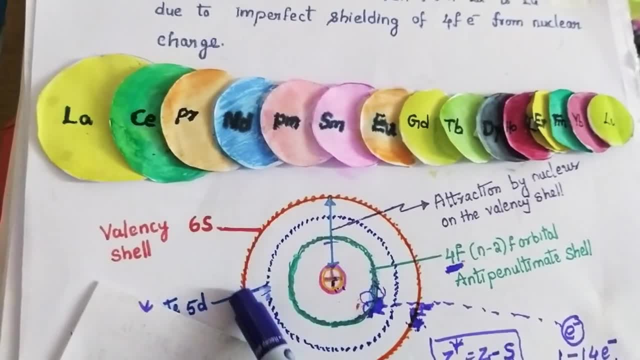 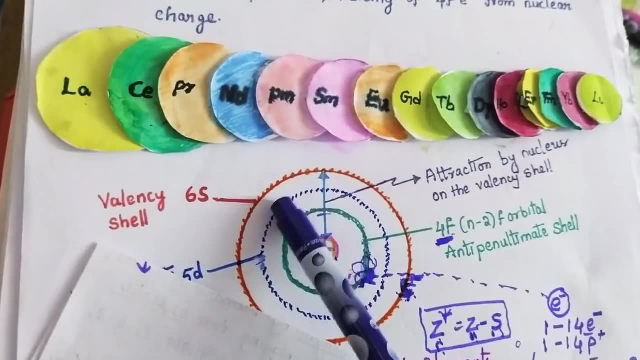 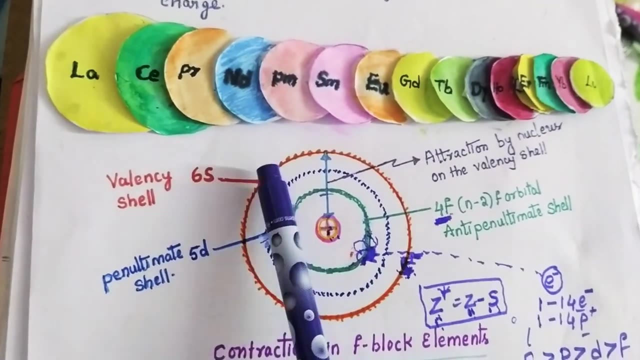 we notice the valency shell that is 6S. valency outermost shell: this is 6s and next to the valency shell that is 5d. so you can notice this is a fifth orbit. so it is consisting 5d. so 6s is consisting common for all that is two. 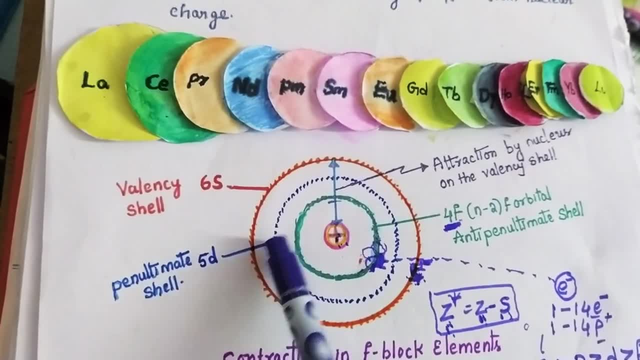 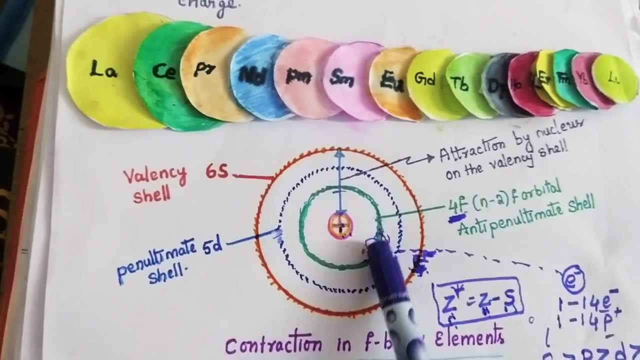 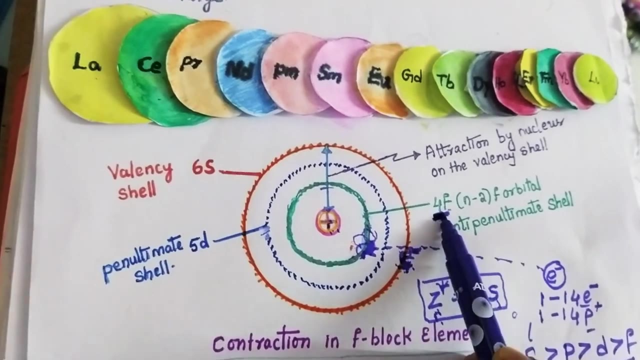 electrons and 5d is consisting either one or zero electron. this is a next to the valency shell, that is penultimate shell. and next, inertial is anti-penultimate shell, that is 4f. right, so this is the 4f. this is the anti-penultimate shell, so the all the electrons are entering into the. 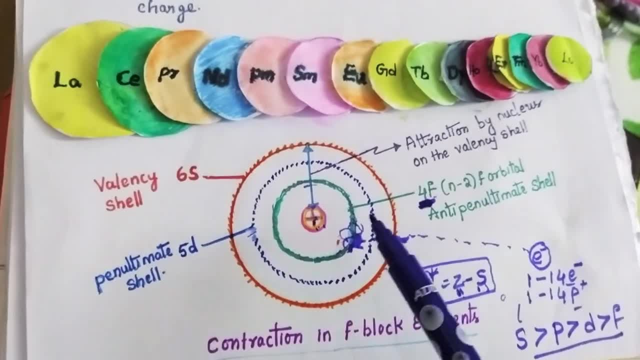 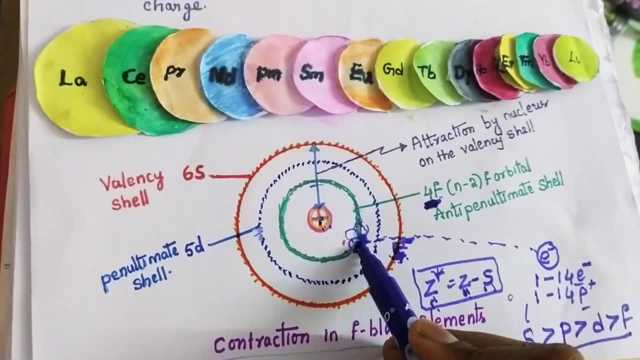 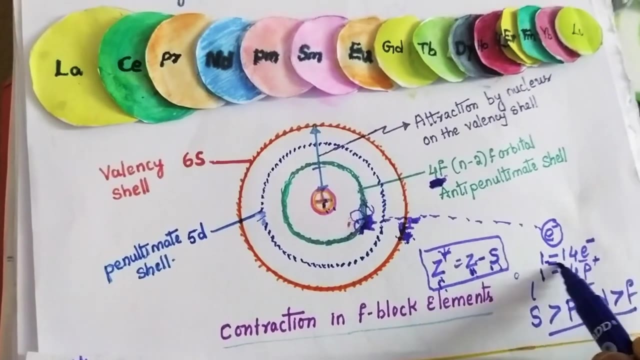 anti-penultimate shell in the f block right. so in the lanthanum there is no f electron but cerium. it is having one electron it is going to enter for cerium and prosodium, neodymium. it is gradually increases: 3, 4, 5 up to 14, so as the number of electrons increases from lanthanum to lutetium. 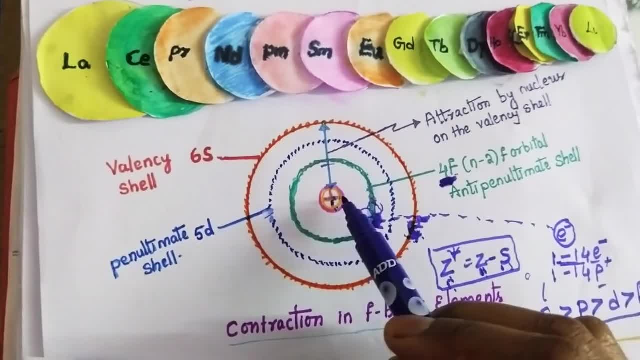 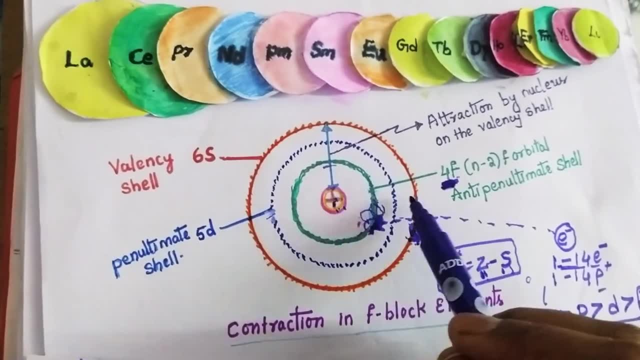 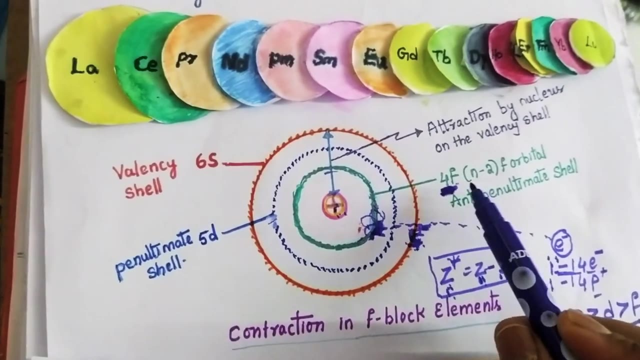 gradually the number of protons also increases. automatically the nuclear charge increases towards outermost electron. the effective nuclear charge also increases. notice here one thing: the number of which electrons are increasing, from lanthanum to lutetium, f electrons right 1 to 14, so f electrons is having 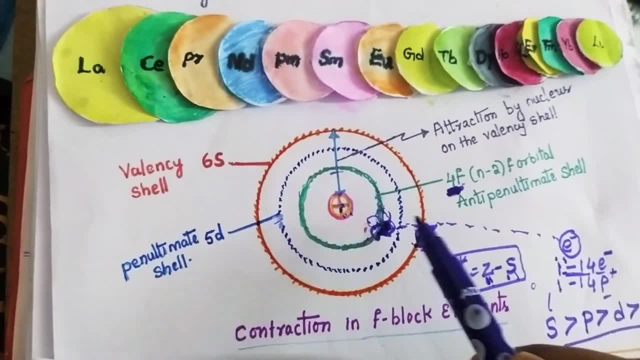 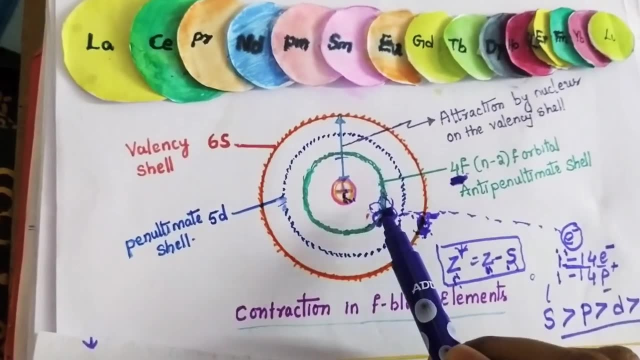 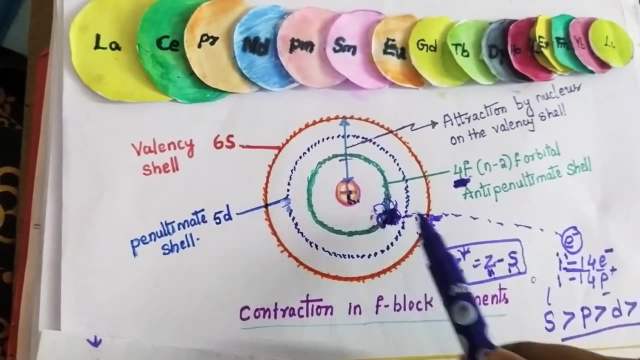 a diffused kind of shape means it can't protect nucleus outermost electron from the nuclear attraction, so it is having poor shielding capacity. so due to poor shielding capacity of f orbital electrons, so the nuclear attraction towards outermost electron will becomes greater and greater. so this is the reason as the number of electrons increases. 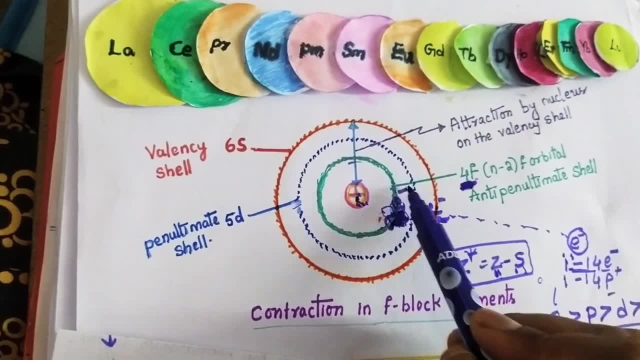 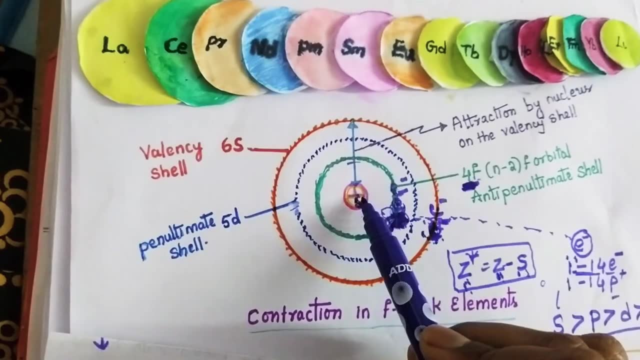 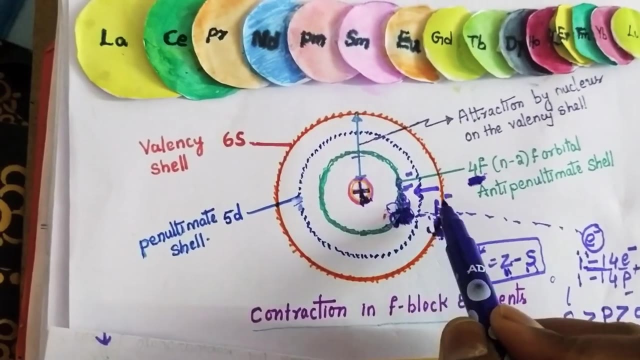 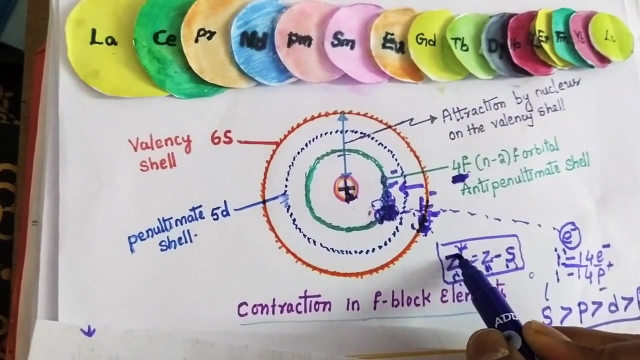 so automatically. so the electrons are entering into the innermost shell, that is a anti-penultimate shell, and protons also increases. so proton increases and effective nuclear charge towards outermost electron increases gradually. the size is going to increase and the number of electrons is going to decrease. it shows some contraction. so what is mean by effective nuclear charge? 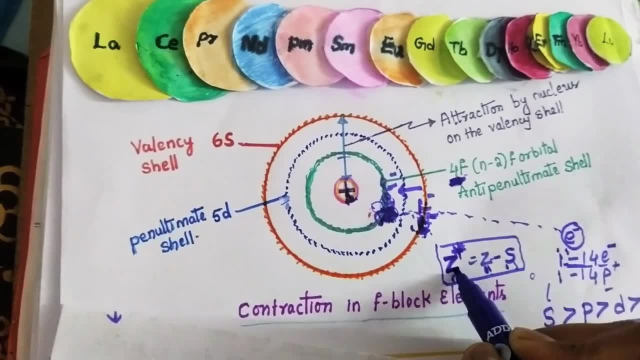 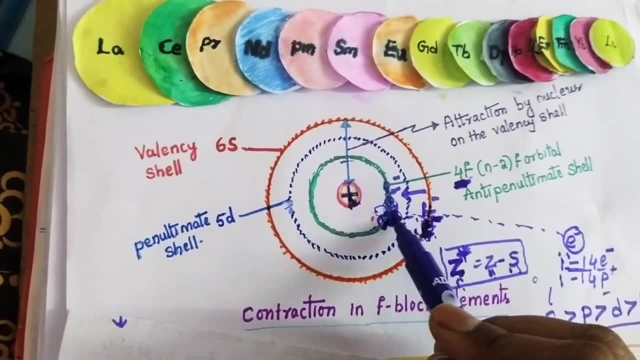 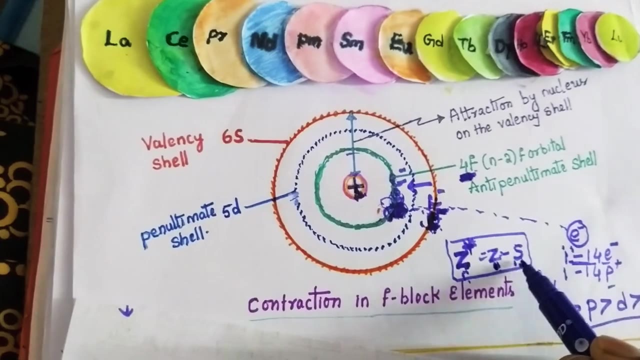 the z星, the effective nuclear charge. that means the actual charge which is getting by the outermost electron. so here, because of shielding capacity it may be reduced. so that can be calculated z minus S. z means Atomic number, s is a shielding capacity between these two orbits, but as I said, the f orbital is having much less oxygen. so i concluded here that you can see that z is an Whose、s. 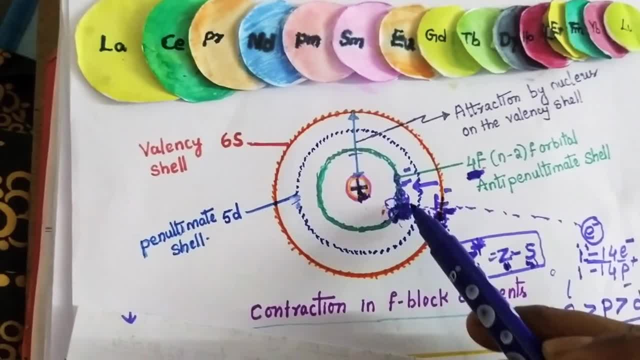 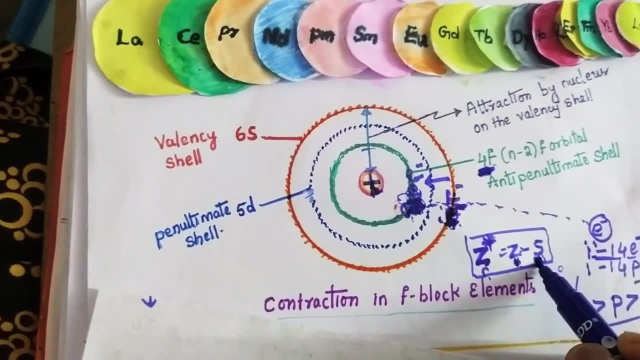 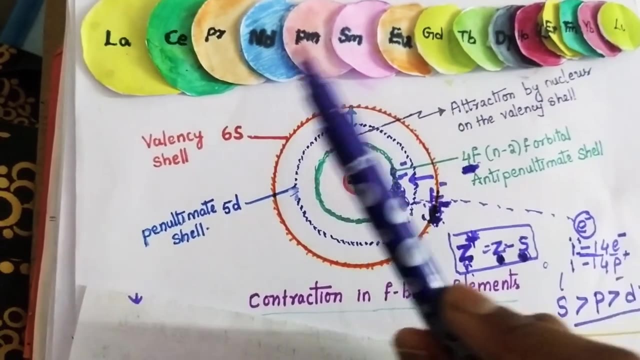 having diffused kind of shape, right. so due to diffused kind of shape, the F orbital electrons are having very poor shielding capacity, so you can neglect this term. so that's why the Z star will become Z, that is atomic number. from lanthanum to lutetium, atomic number increases. 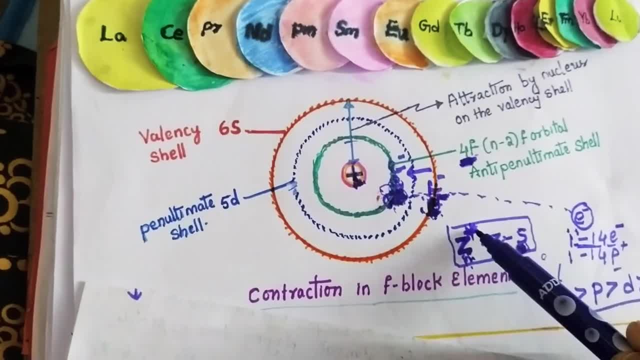 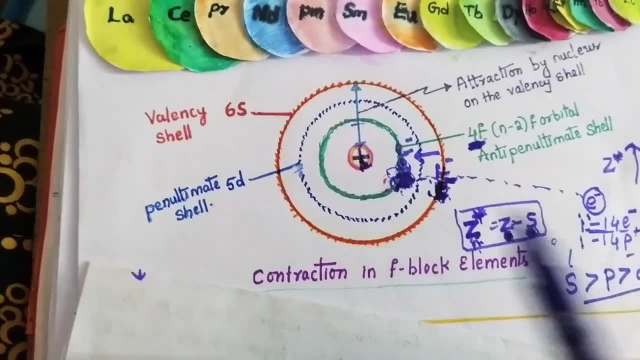 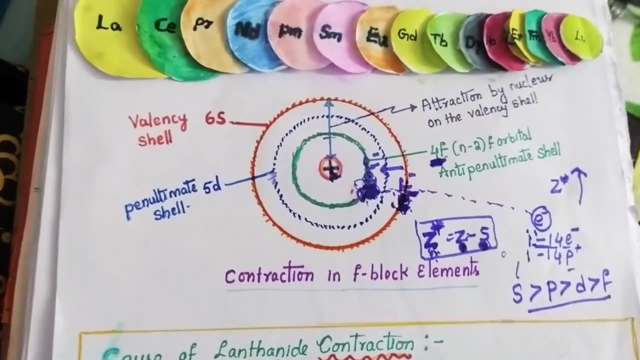 from 57 to 71, automatically the effective nuclear charge, that is, Z star, also increases. so this is the way. this is the reason for the lanthanide contraction, right? so the lanthanide contraction we can define one more time. so here you can notice. 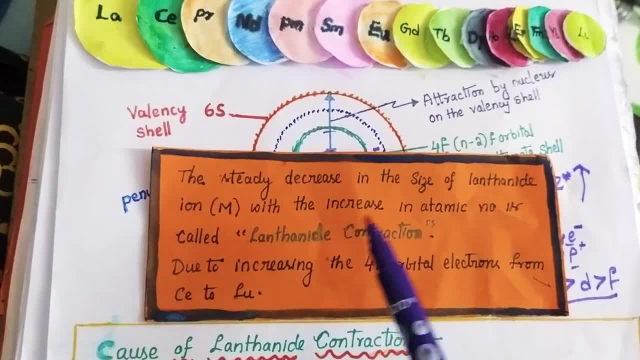 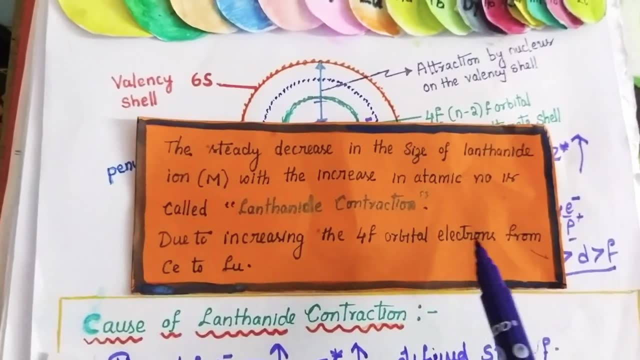 the study. decrease in atomic sizes of lanthanide ions with increasing atomic number is called lanthanide contraction. this is due to increasement of number of 4F orbital electrons from cerium to lutetium. is this clear? so next we are going to see what are the. reasons for the increase in atomic sizes of lanthanide ions. so this is the reason, the reasons I already discussed. we are going to write one more time the first reason. first reason: as number of 4F electrons increases, so 4F electrons are having poor shielding. 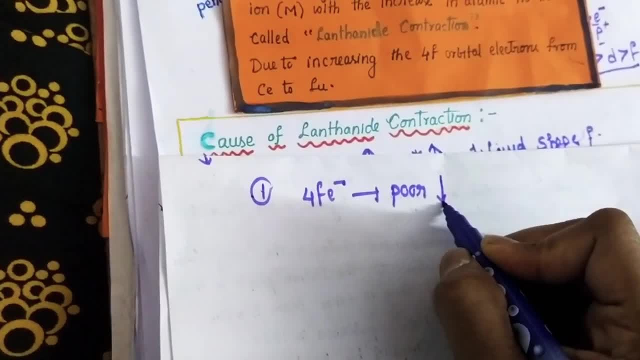 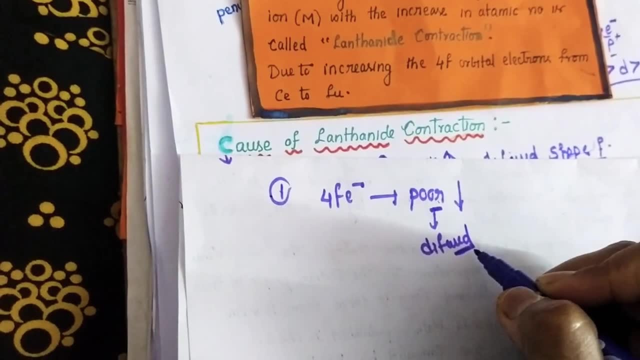 capacity, that is a poor screening capacity. so, due to poor screening capacity. why poor screening capacity? because it is having a diffused kind of shape. it can't protect properly the outermost electron from the nuclear attraction as number of 4F electrons increases. 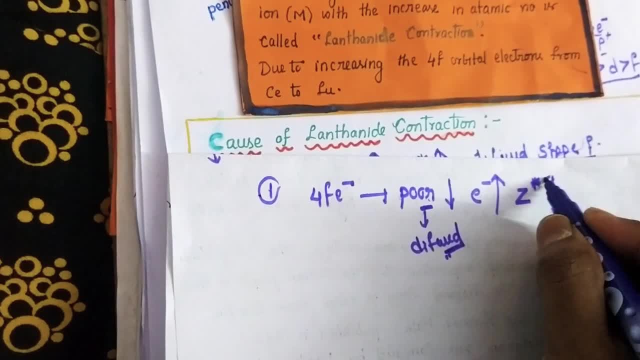 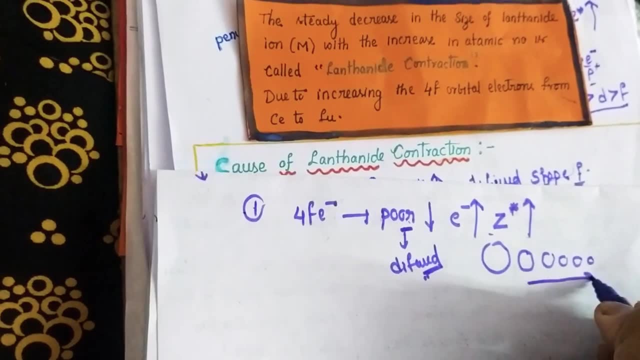 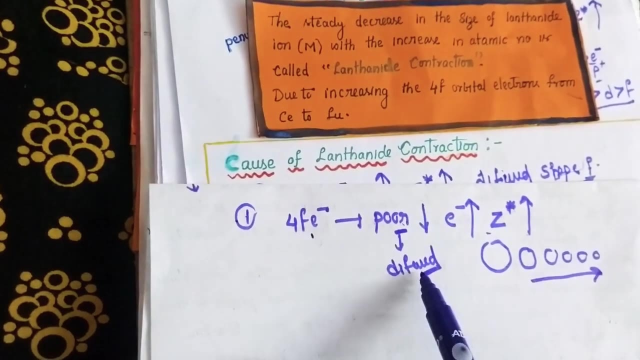 gradually the Z effective atomic number also increases and size gradually going to decreases, so this is called as lanthanide contraction. the main reason is due to the poor screening capacity of 4F electrons because of its diffused shape and Z effective atomic number gradually increases. 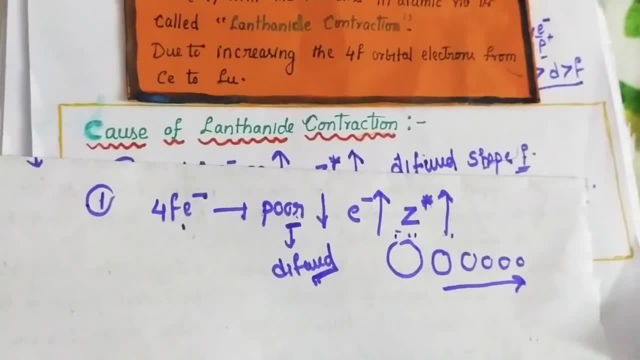 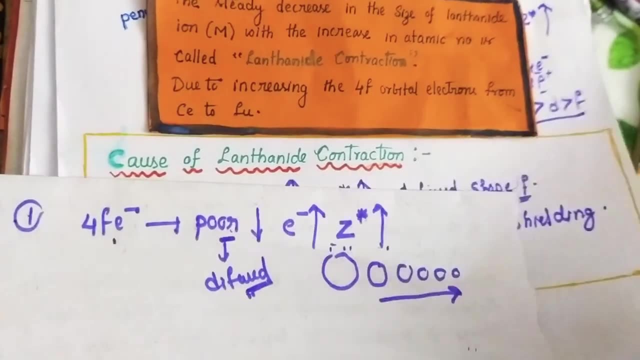 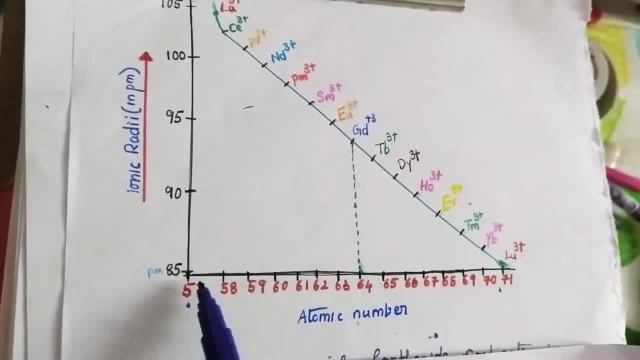 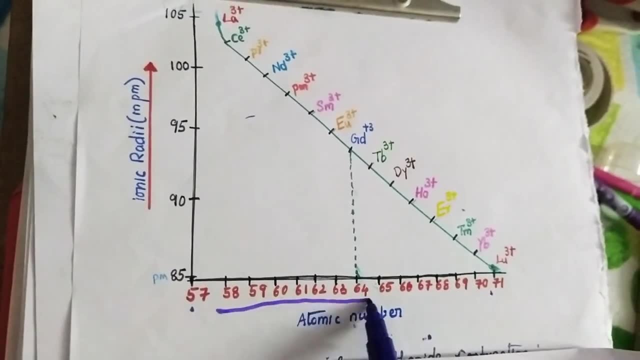 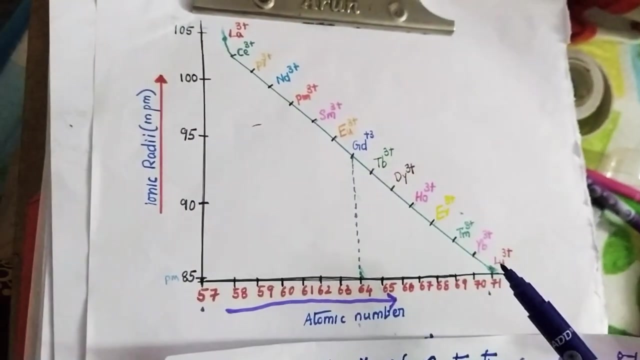 to represent. see here in this graph. so this is the atomic number of lanthanum to lutetium, that is, 57 to 71,. as atomic number increases, what is going to happen? so the ionic radii is gradually decreases from 105 to 85 picometer. right, we have to notice. 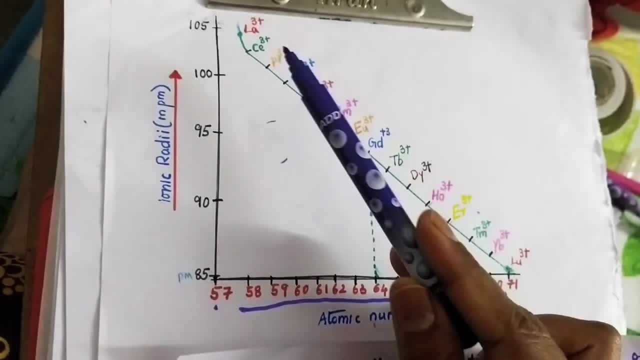 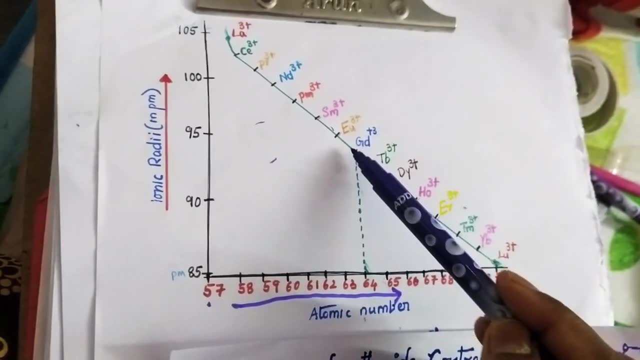 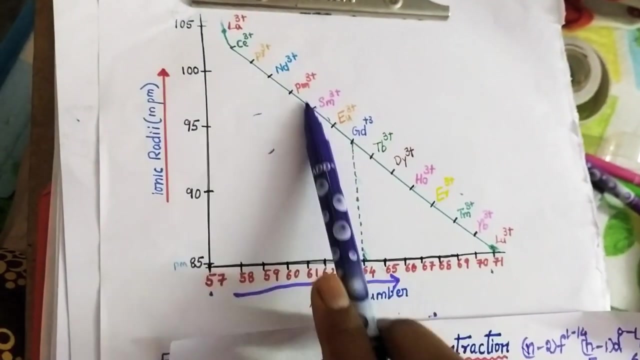 here one thing. so this is a picometer. if you make it average, each element atomically, atomic radii is gradually decreases around 1.5 picometer. that means there is a regular decreasement of atomic radii from lanthanum to lutetium. so this decreasement is because of 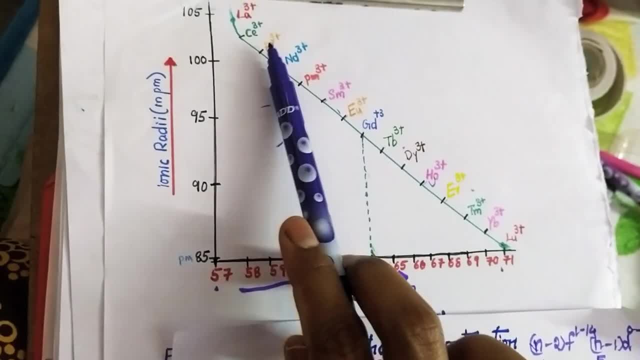 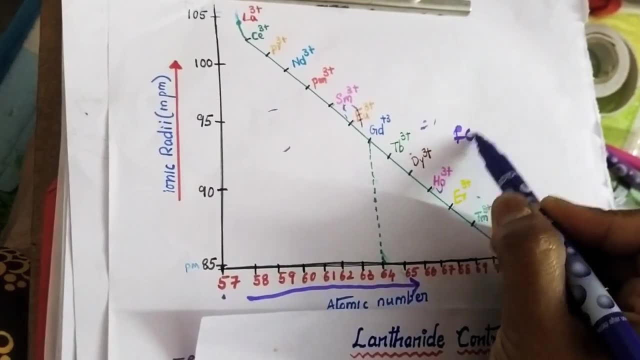 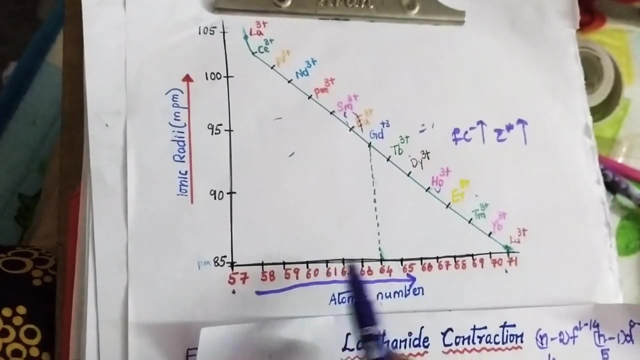 number of electron because each element is getting one more F electron. as one electron increases, one Z star will increase, so F electrons are increasing automatically. effective nuclear charge also increases, right? this is the graphical representation. from this you can understand how the lanthanide 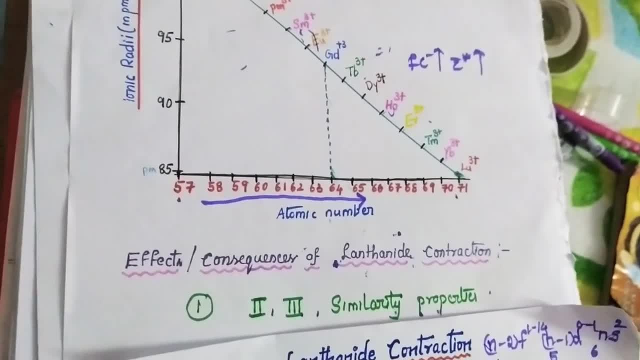 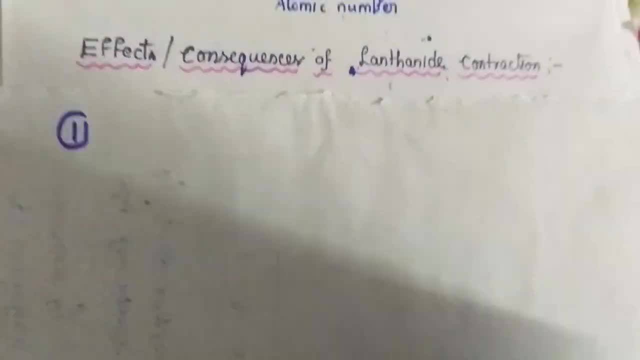 contraction is happening. so next, what are the effects and consequences of lanthanide contraction? the first consequence is: see here the lanthanides in the periodic table where it was located here. so this is the lanthanides it was located around, that is. 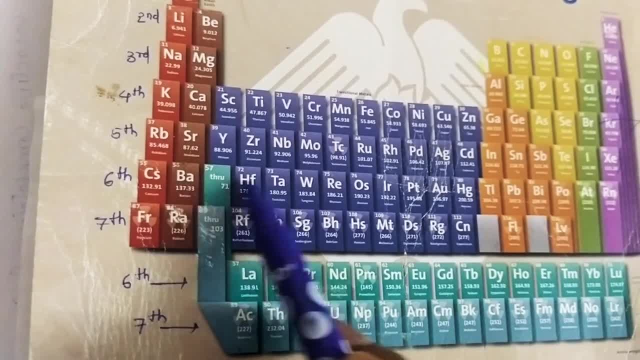 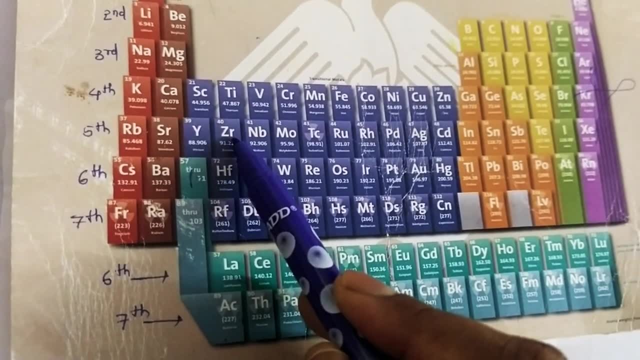 a third series of transition element. this is a first series, second series, third series. here lanthanides are noticed right. due to this lanthanide contraction, the second series of transition elements shows similar properties with the third series. you know that group. 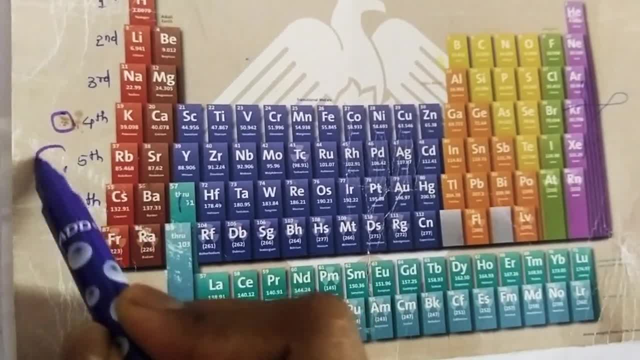 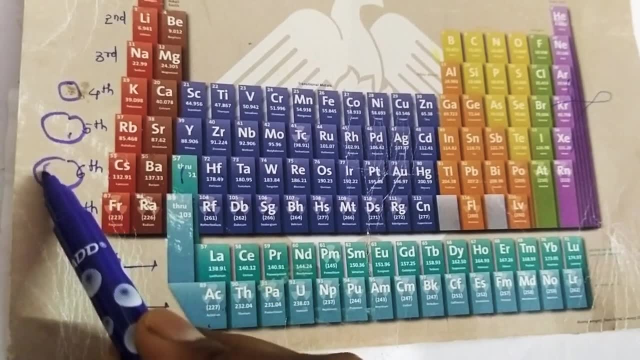 sizes gradually increases. that means from here to here, here to here, here to here size will increase, but here gradual increasement rather than increasement. there is a decreasement is happening because of lanthanide contraction, so it will become almost equal size. so that's. 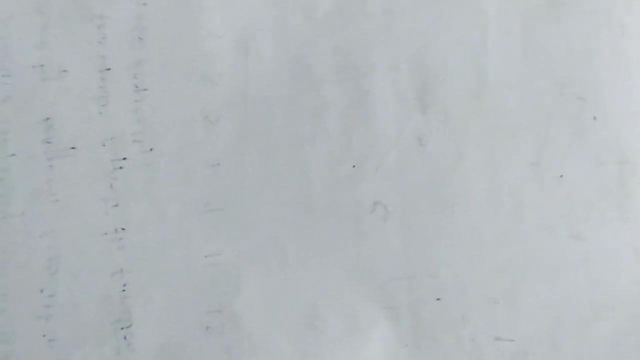 why there is a similarity in the properties of zirconium and hafnium, so the first consequent is the zirconium and hafnium. they are the ones that are at equal size. so these are the shows similar in the properties because of its lanthanide contraction. the second consequent is from lanthanum to lutetium. the size is decreases. right, as we discussed here, the size is decreases. so when size decreases, what will happen? when size decreases automatically, size decreasing means the nuclear charge will. 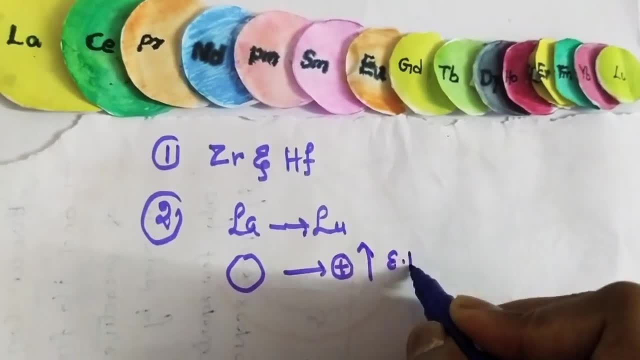 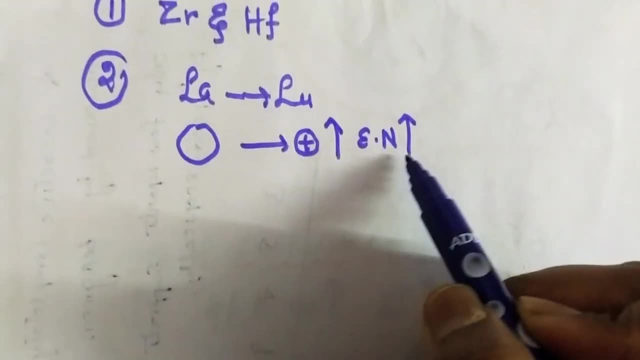 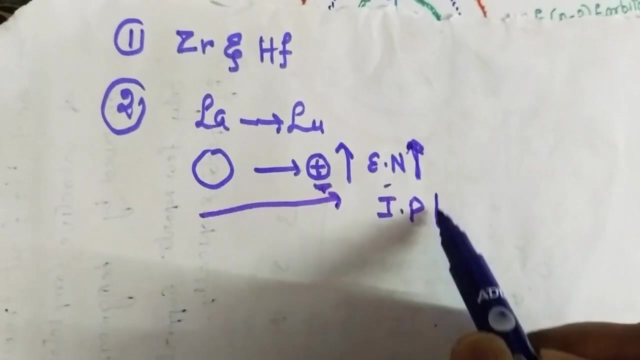 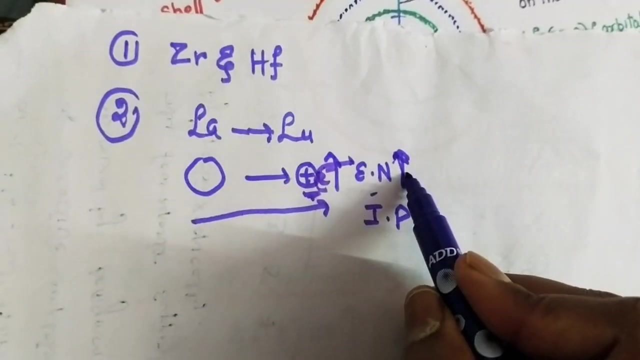 increase. charge increases means the electronegativity increases. electronegativity means the electron accepting capacity. electron accepting capacity also increases and also size decreases means the IP value. that means ionization potential. that means the energy required to remove outermost electron is also increases. electronegativity increases IP increases. 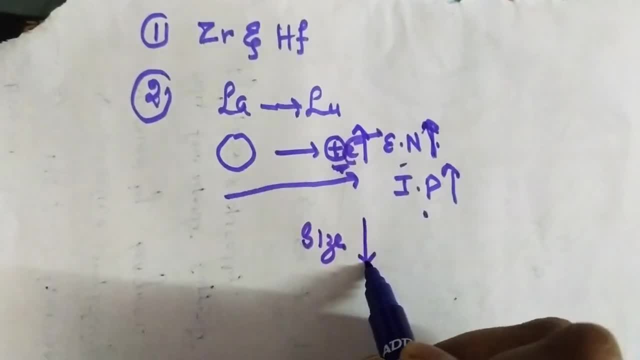 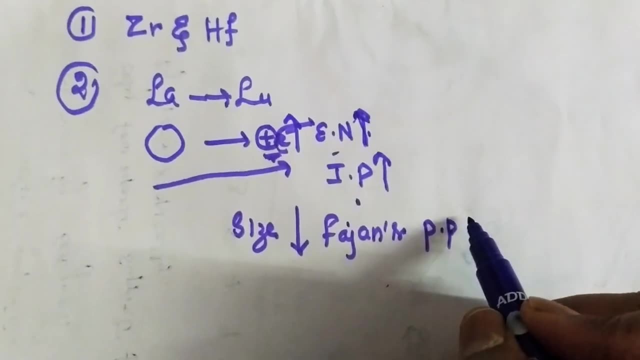 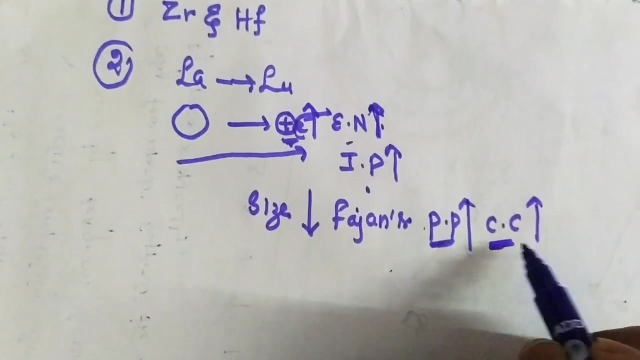 at the same time, cation size decreases. according to Poisson's rule, the polarization Polarizability- that is, a polarizability of cation- sorry, polarizing power of cation- increases, covalent character also increases. So we know that covalent character increases.